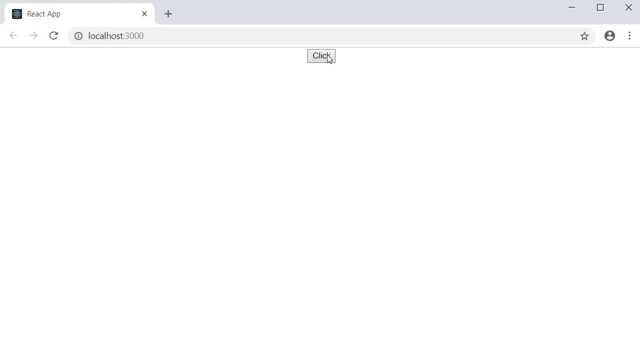 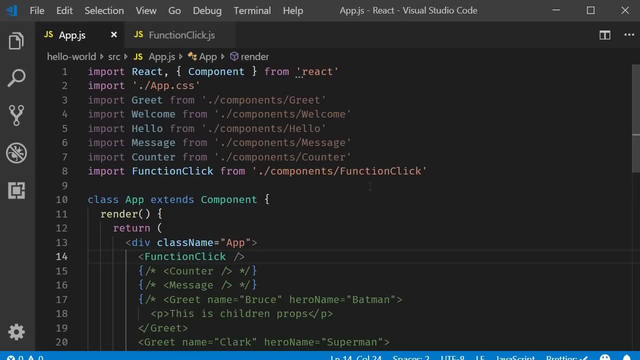 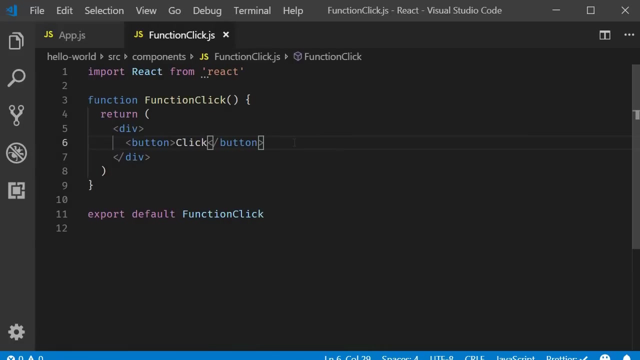 click event and execute some basic code. The first point you have to make note of is React. events are named using camel case rather than lower case. In plain HTML, In the JavaScript you would specify onClick, but in React it has to be camel-cased. so 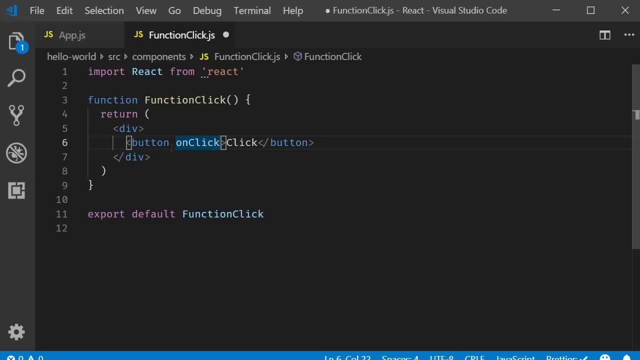 C has to be uppercase onClick. The second point is: with JSX you pass a function as the event handler rather than a string. So instead of clickHandler within double quotes, you are going to have clickHandler within curly braces. Now let's define the clickHandler function. 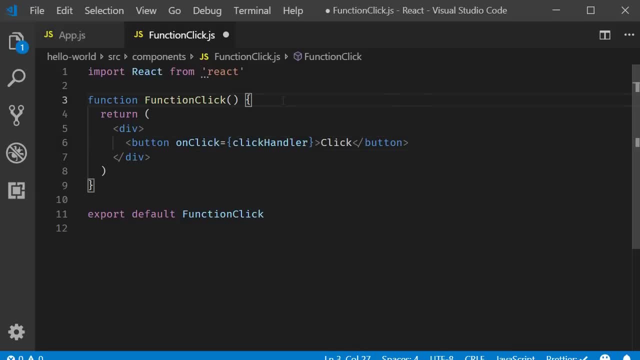 Remember, in JavaScript it is very much possible to define a function within another function. So inside the functional component we can define our clickHandler, So function clickHandler, and within the body we simply log to the console buttonClicked. Let's save this and test it out. 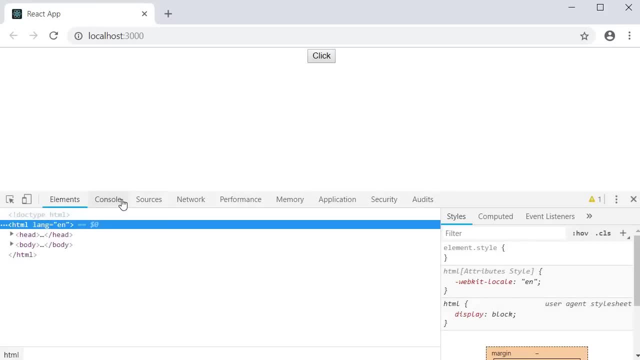 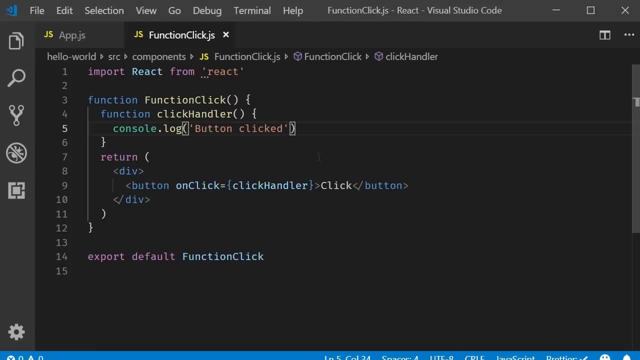 If I open the developer tools and the console tab and click on the button, you should see the message buttonClicked in the console. Our click event handling works as usual, As expected. Now let me point out one of the more common mistakes we, as beginners, tend to make with. 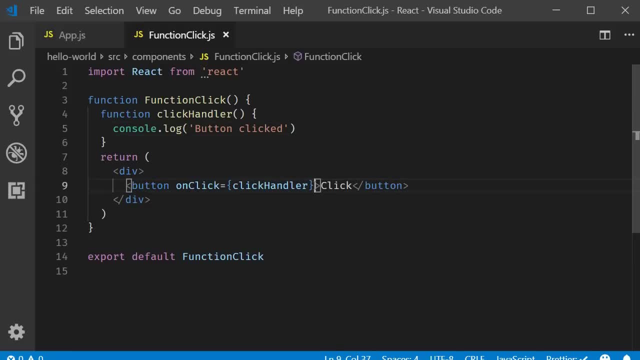 event handling. In our code you can see that onClick, we pass the function as the event handler. Pay close attention to the absence of parentheses. If you do add parentheses, it becomes a function call, And that is not what we want. 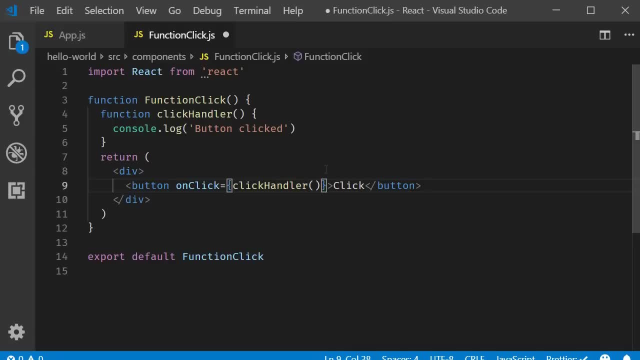 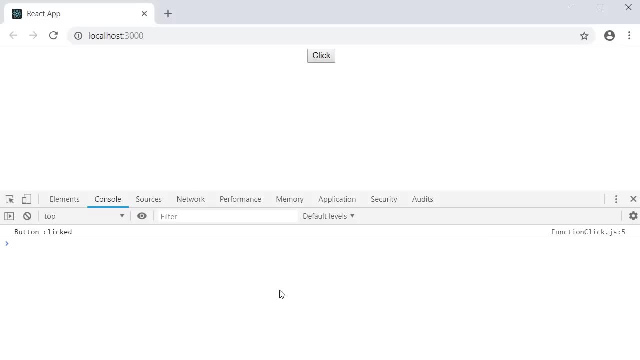 We want the handler to be a function and not a function call. Let's quickly see what happens if we do leave the parentheses. I'm going to save this and go back to the browser And you can see that in the console the message buttonClicked is already logged. 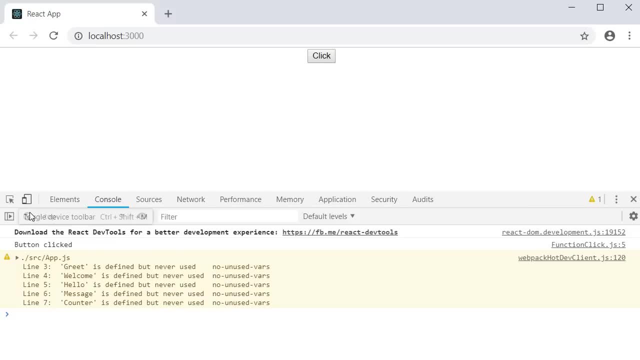 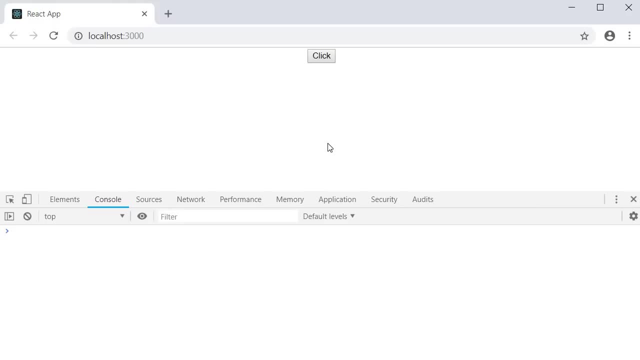 Refresh, Refresh. The message is logged in the console. Now this scenario becomes worse in class components. when your click handler changes the state of the component, The component constantly re-renders and you might see an infinite number of messages in the console. 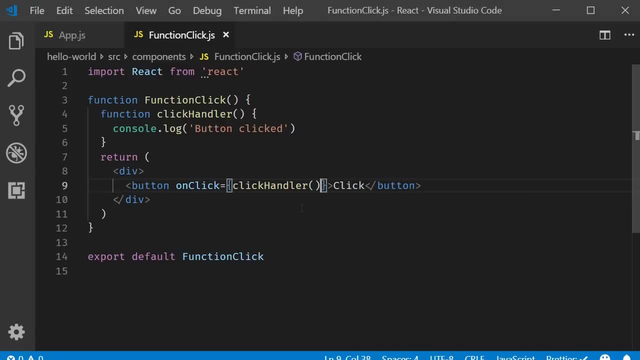 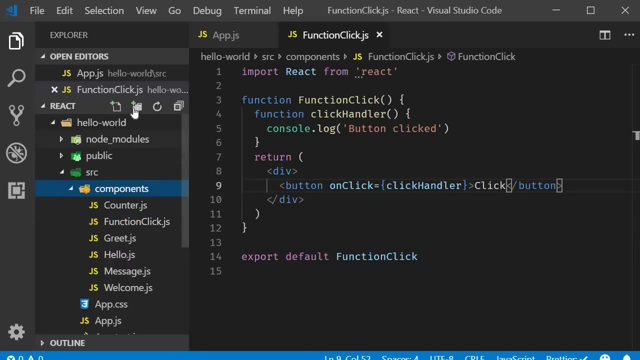 So what I want you to keep in mind is that the event handler always changes the state of the component. handler is a function and not a function call. Do not add the parentheses, Alright? next, let's take a look at event handling in class components I'm going to create. 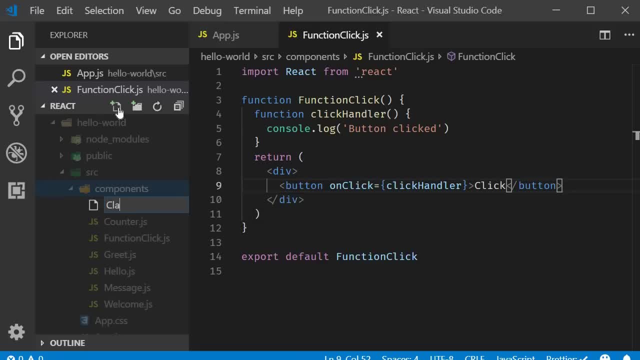 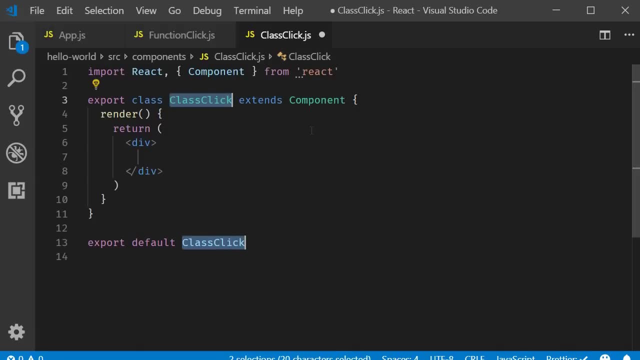 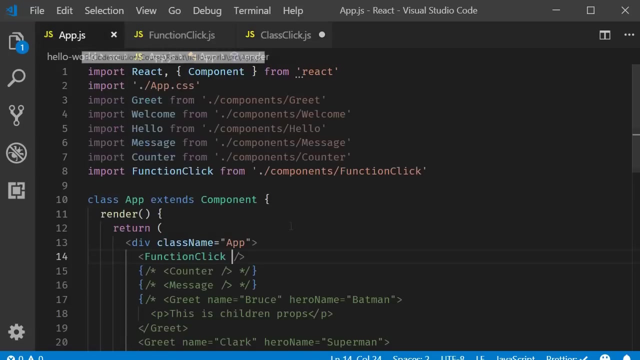 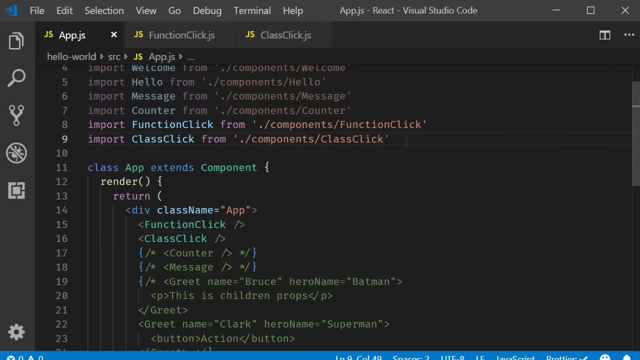 a new file called class clickjs and within the file I'm going to use the react snippet RCE to create a class component. I will get rid of the named export and include the component in app component. Again, make sure you import the component at the top In the class click component. 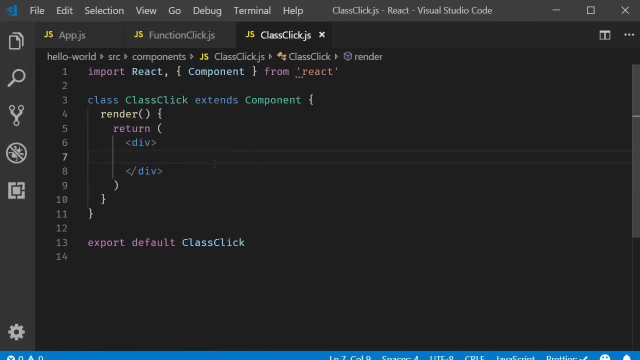 JSX. I will simply add a button with the text click me. If we take a look at the browser, you should be able to see the button Now. adding a click event handler in a class component is very similar to functional component. We have the onClick attribute. 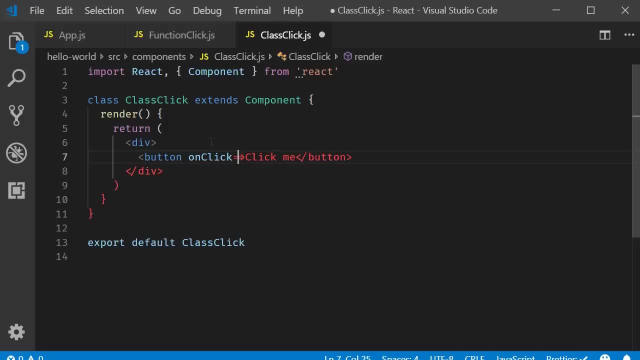 in camel case, of course, and this is going to be equal to curly braces and within the curly braces the handler. But in a class, component methods will be accessed using the this keyword, So this dot click handler. Now we can define the class. so, right above the render method, click handler and we simply log to the